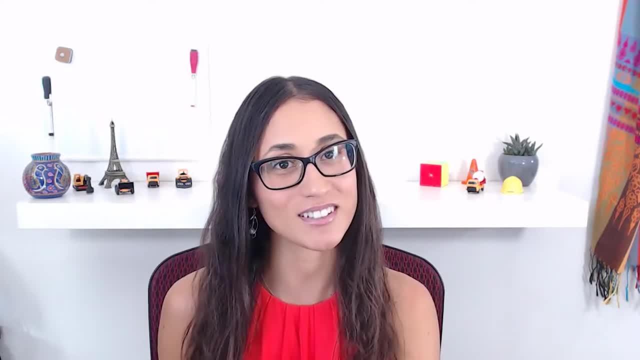 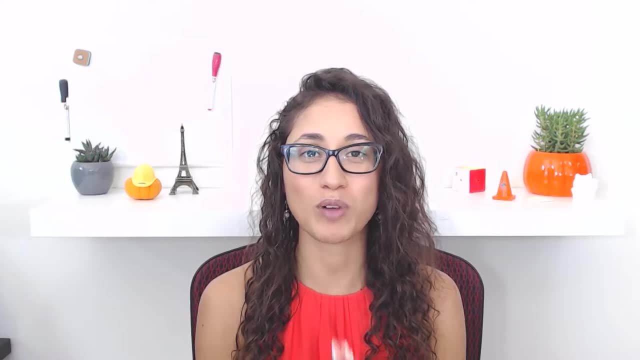 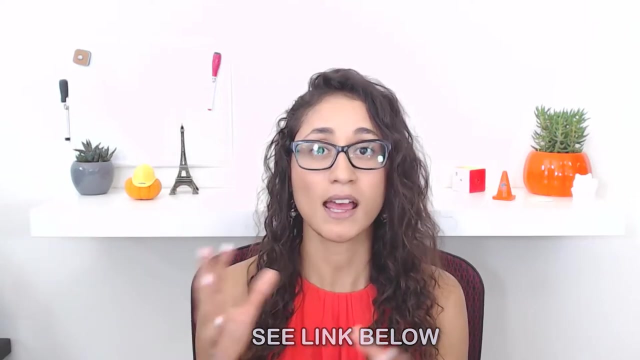 bell, so you don't miss out on future videos. Now let's get started. Okay, guys. so in this video we're going to cover problems using AASHTO. This is the second part of the first video, where we covered problems using USCS. As I mentioned before, I split this video into two parts. 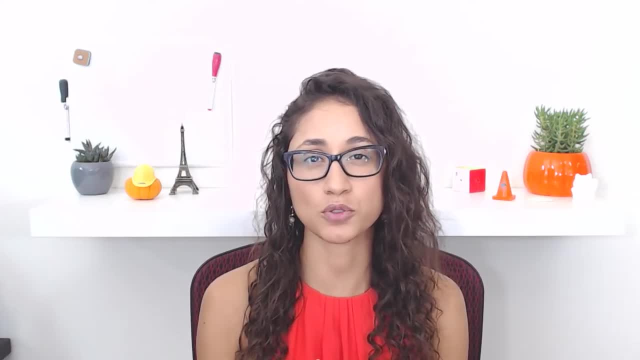 because it was a little bit too long and I like to keep the video short, so that way you focus and grasp the material better. Now don't forget to do the problems with me as you go, because the best way to learn something is by doing it. Question number seven: Using AASHTO. 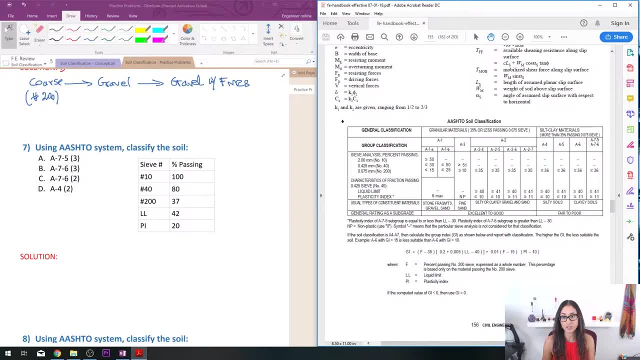 system, classify the soil. So we have percentage passing- Again, the same thing as the USCS. the first thing you look at is the sieve number 200. Now here it is giving us 37%. that's passing. This is actually easier, AASHTO. They only use one term, which is passing. They even show it with the 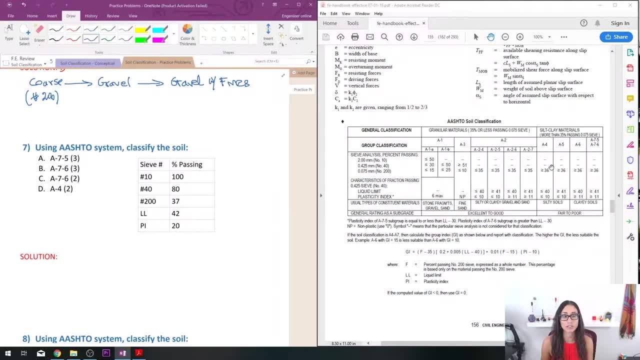 signs. So for these categories it has to be greater or equal to 36, and then for here it's less than or equal to 35. So on this we have 37. That means that we have less than or equal to 35.. 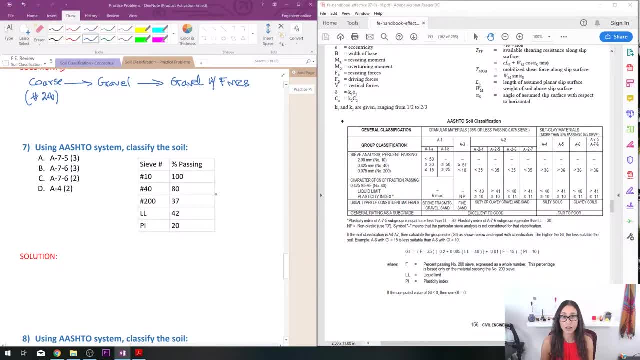 So on this, we have 37. That means that we have less than or equal to 35.. So on this, we have 37. That means it's greater or equal to 36.. So it's going to be any one of these groups right here. 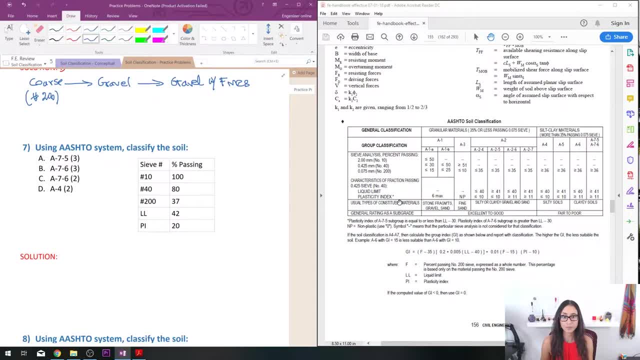 After that we're going to look at the liquid limit. So my liquid limit here is 42. So that's going to be either A75, A76 or A5, because it's all greater than 41. It has to be greater than 41.. 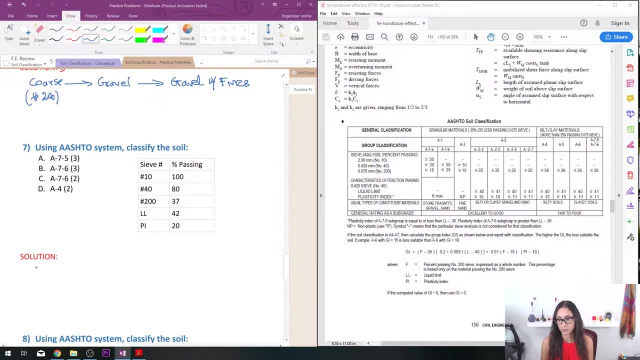 So let me, let me write it down. So we have. so first we said it's going to be silt clay, because it's greater than this. we determined this from the 200 sieve, and then we said it's going to be either A5,. 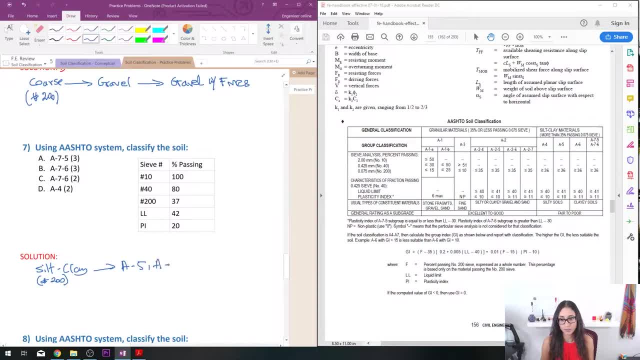 A75 or A76.. Right, Because the liquid limit is greater than 41.. okay, now, after determining that, then now we're going to look at the P I. so P I here notice that we don't need to calculate anything because P I is. 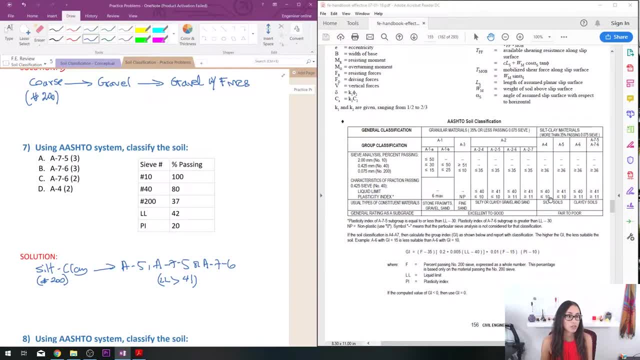 already given it's equal to 20. so the P I here it has to be less than 10. so I already know that a 5. I'm going to cancel it because my doesn't satisfy my P. I now P. I here a 7, 5 and 8, 7, 6 is greater than 11. so that works. but which? 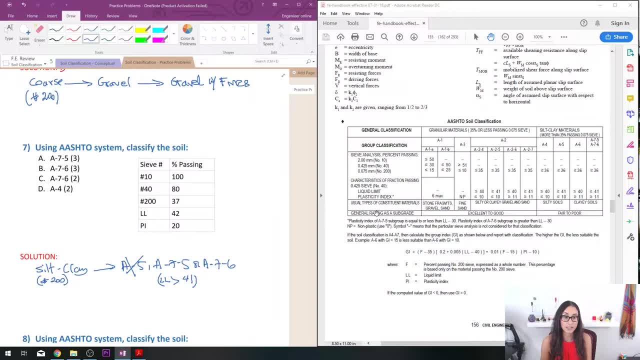 one. is it a 7, 5 or 8, 7, 6? if you look at down here, it gives you that if it's equal to, if the subgroup or the P I equal to or less than L liquid limits minus 30, then it's a 7: 5, but if it's greater than we have a 7: 6. so my P I is: 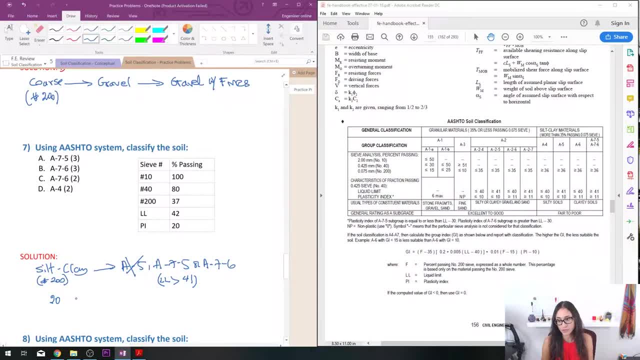 20 and I have to see. so I have 42 minus 30 and this is equal to 12, right? so 20 is greater than 12. so if it's equal to or less, so that doesn't work. so it's greater than right. so I have a 7: 6, so that's gonna be 8, 7, 6. that's my answer. 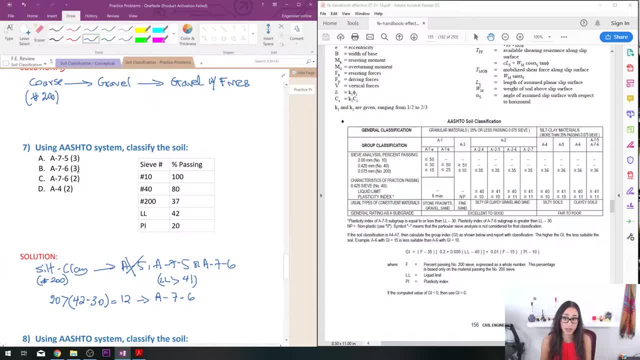 but I still need to calculate the GI. so I already know the answer is going to be either B or C, or I'm just going to have to do it again. I'm going to have to do it again, or C, but I need to find the GI for to be able to answer the question. so my GI is: 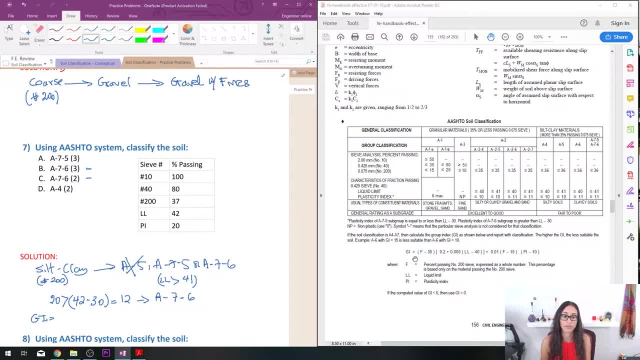 equal to. so this is the equation is right. here we have F. F is just your percentage for number 200, for seed number 200. so I have 37 minus 35, and then we're going to do times 0.2 plus 0.005, times you liquid limit, which is 42 minus. 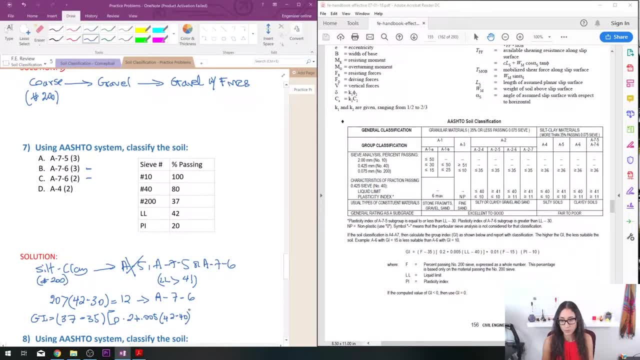 40. we're going to close the parentheses. then we're going to add 0.01 times F, which is 37 minus 15 times the PI, which is 20, and then we're going to add 0.01 times F, which is 37 minus 15 times the PI, which is 20. 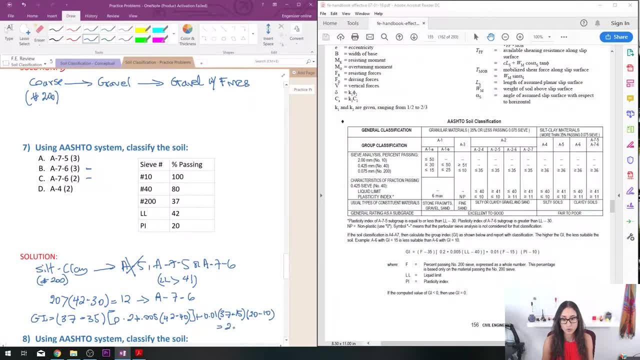 minus 10. now this gives about 2.62. but remember one of the rules for GI is that you already always have to round up. so if it's 2.62, we're going to round it up to 3. so your answer is going to be B a, 7, 6. with a GI of 3, problem 8: we have 45%. 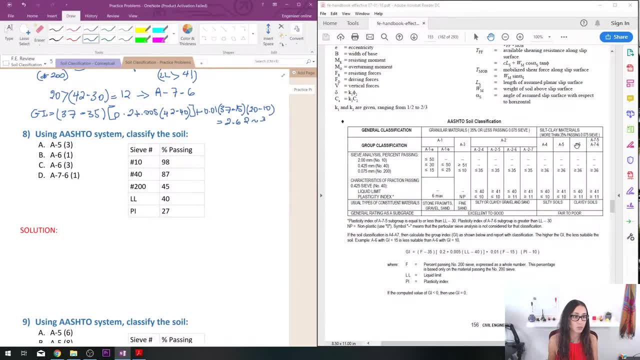 passing seed number 200, so that's going to be anywhere under this category: either eight, four, five, six or seven. let me write that down. so it's going to be a four, two, a seven. after that we have liquid limit of 40, so it has to be equal. 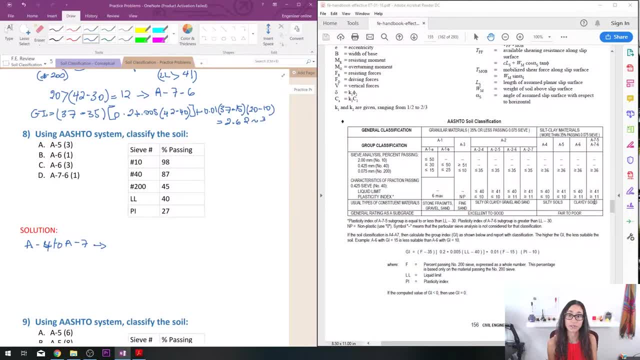 to 40. so a five and a seven don't work. so which is? it's gonna be either a4 or a6. so either a4 or a6. this is a because of the liquid limit is equal to 40. so next we need to determine the plasticity index. 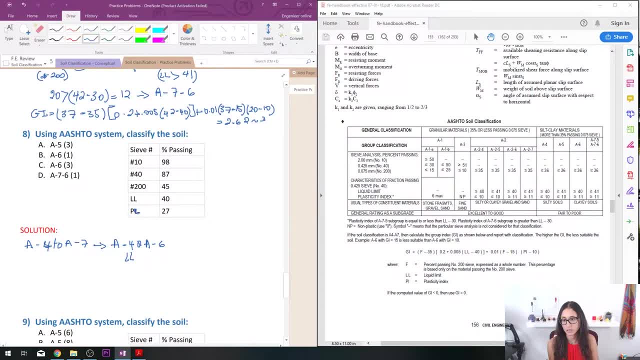 this is actually a pl. that was a mistake. okay, so pi would be equal to 40 minus 27, which equals to 13. so once you determine your pi, then we can see which group it is. so we have 13. so that means it's greater than 10 or greater than 11. so that's going to be a6. so our answer: 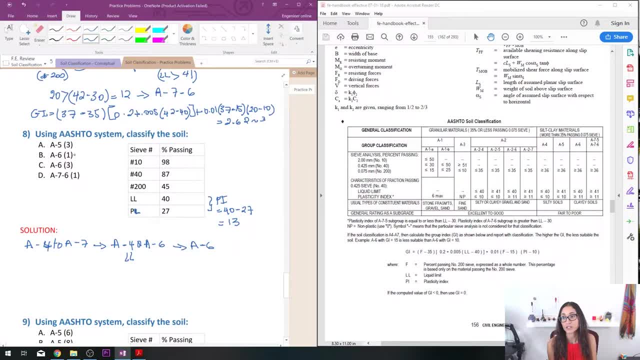 it's going to be a6, so it's either b or c. we still need to calculate gi. so gi, so it's going to be f, which is the percentage passing 200 sieve. so i have 45 minus 35 times 0.2 plus 0.005 times my liquid limit, which is 40 minus 40. so notice that this is going to be. 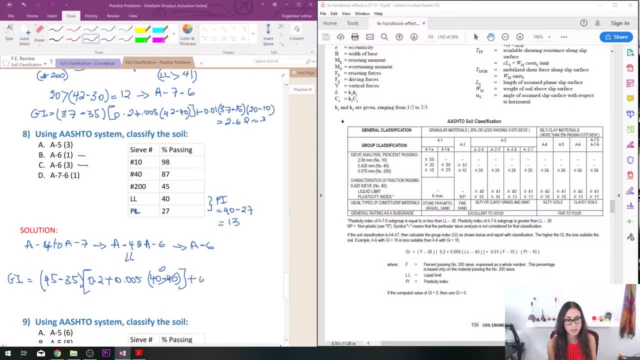 zero plus 0.01 times f, which is 45 minus 15 times pi, which is 13 minus 10, which equals to 2.9. so remember, we always have to round up, so that's going to be equal to 3, so our answer is c. 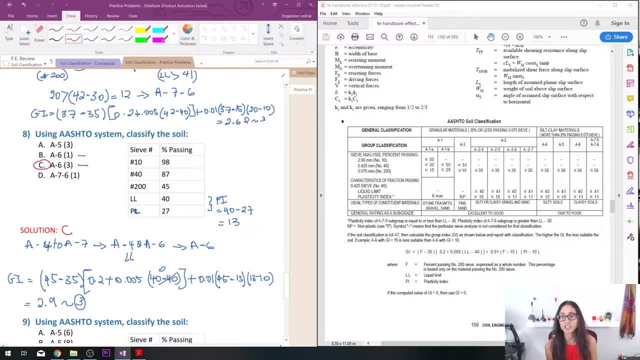 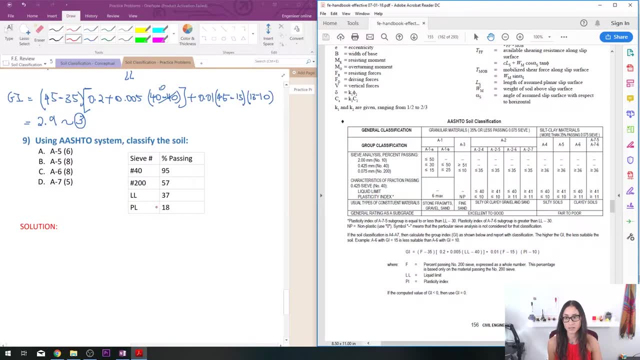 a6 with a gi of 3. okay, last problem. so we have again similar. so we're going to look at sieve number 200. so we have 57 percent. that's passing. uh, again, it's going to be under uh, these categories between a4 to a7, so let's write it down: a4, we change color. 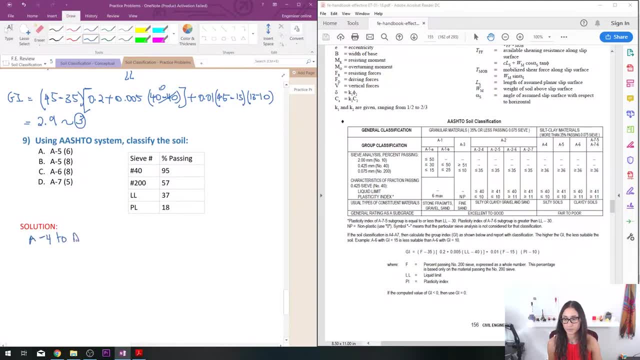 a4, a7 to a 7. then we are going to look at, uh, our liquid limit, which is 37, so that's going. so that's less than 40 um. so it's going to be either a4 or a6- sorry my bad, a6- and then after that we are going to determine. p. i again we're going to ask: uhm. so after that we are going to, vous're going to determine pi again. toum, we're going to do pi with violin. in the figure a 4, the positivism should be equal to c pipe, A2 pepperau. 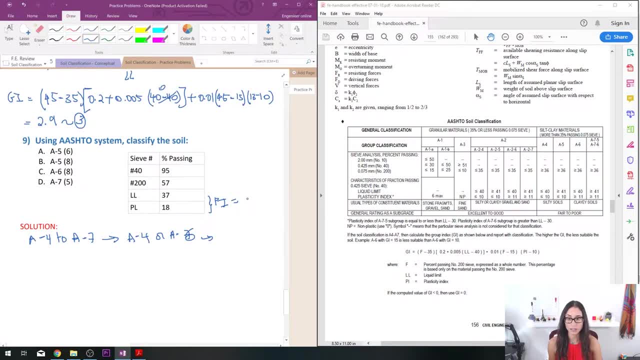 which is 37 minus 18, which is 19.. now, with that, we are so 19, that's going to be greater than 11, so it's going to be a6. now, once you determine that now we need to find gi again, we do the same thing. we do 57 minus 35 times 0.2 plus. 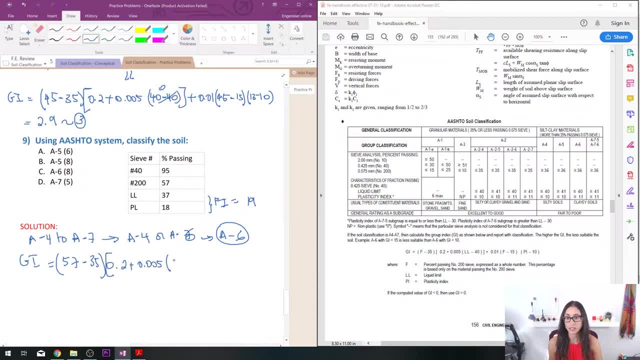 0.005 times the liquid limit, which is 37 minus 40 plus 0.01 f, is the percentage of c 200, which is 37 minus 15 times pi, which is 18 minus 10.. so this should give you 7.85, which will 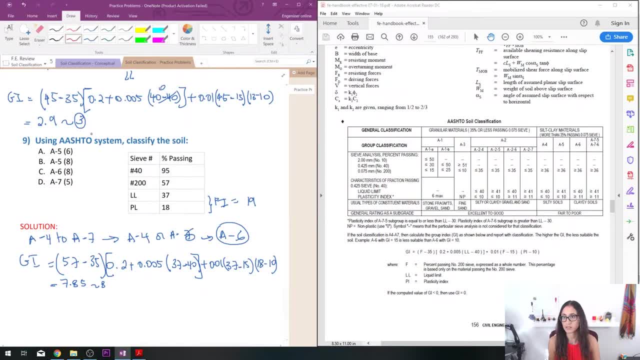 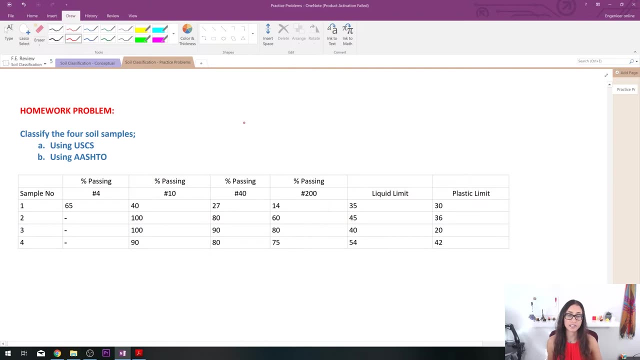 will round up to 8. so the answer is c a6 with a gi of 8.. okay, so for homework i would like you guys to do this problem. um, it's very similar to what we did. so we have four soil samples and um for each sample. you're giving all the data that you need. so the percentage passing for c4: 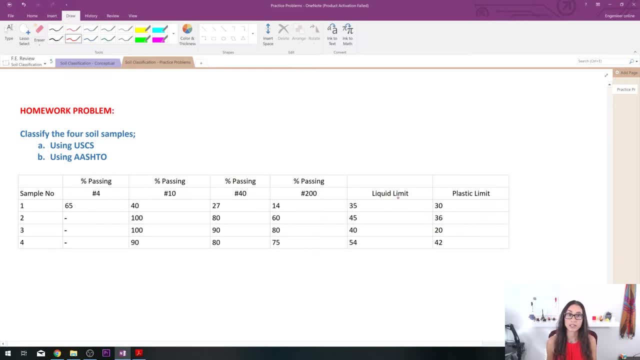 200. sometimes you will need 40 liquid limit and the plastic limit and you need to classify all this sample using uscs and using ashto. once i see a lot of you answered this question, i will post the answer below in the comments, and so hopefully that can help you. uh, kind of see what 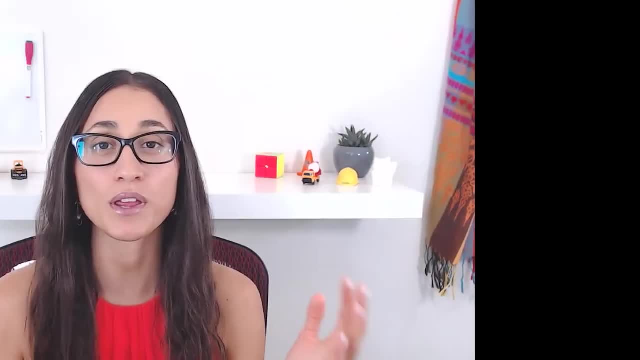 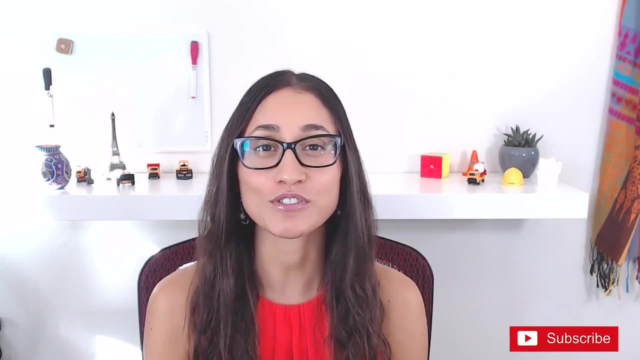 you did and gives you more problems to practice now. if you have any question or is there a specific problem that you would like me to go over, please leave a comment below and i will answer it in the next video in the comments below. don't forget to subscribe, like and make sure to share with your friends. 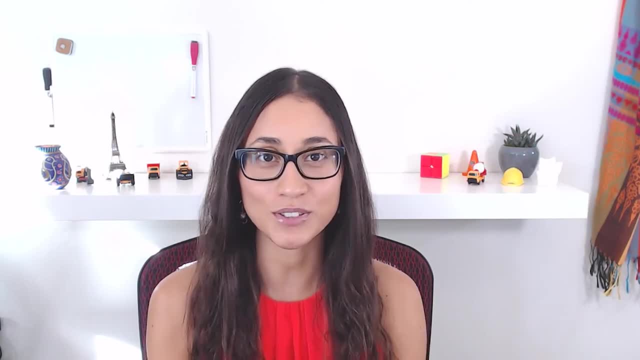 who might find it helpful. thank you guys for watching and i will see you soon.